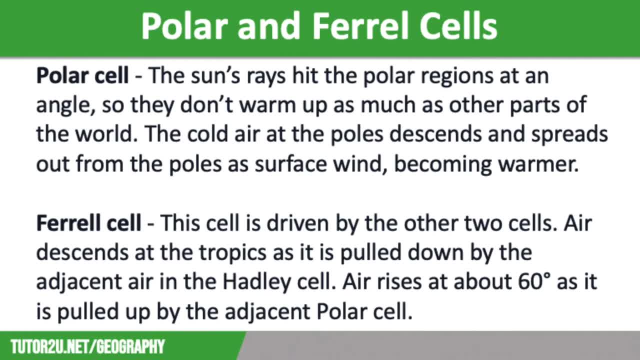 The cold air at the poles descends, meaning there is no condensation and rain. This cold air spreads out from the poles as surface wind, becoming warmer At around 60 degrees. this warm air rises, leading to clouds and clouds. This is when the temperature increases. 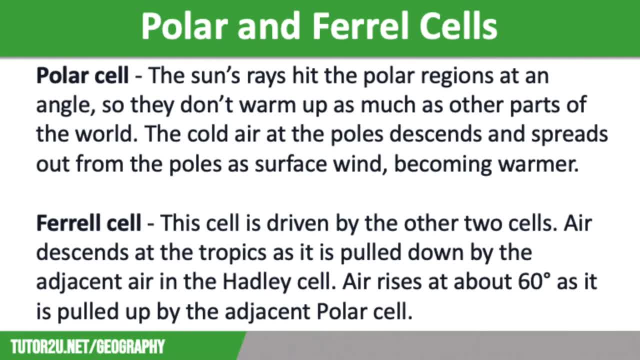 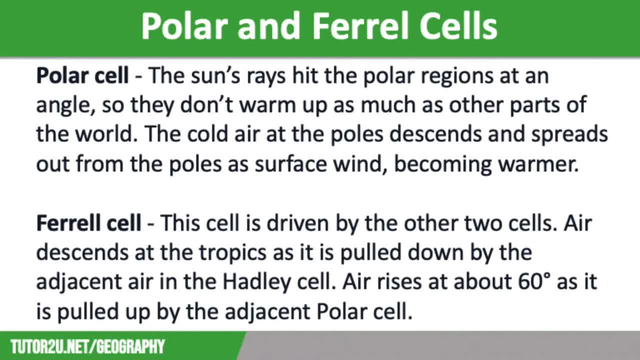 This AIR tends to be very unpredictable. Air descends at some söyes, like the moderates and the centrales, like this one. Thelieux naturally rises across them, shutting off these UV rays. Air descends at the tropics as it is pulled by indirectly adjacent air in the Hadley cell. 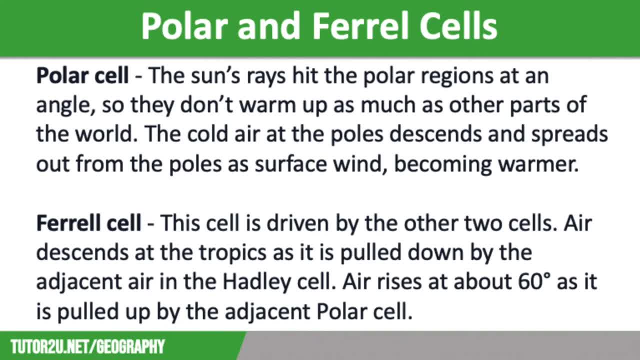 Air rises at around 60 degrees and descends along the B conquest and remains constant to the polar core as it is pulled by the adjacent polar Button. This is how it is in the water at the top, like the right, the left andeyest to build. 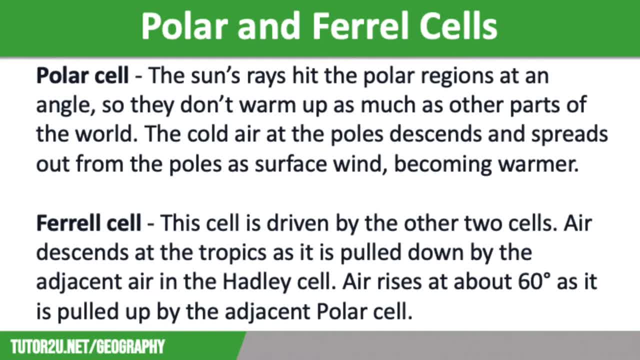 the system – which can move this head up and down. But the water does not Result if it has a vent, because obviously we can't find inspiration. It is difficult for boundaries between the polar air, which is cool. The smallest and weakest cells are the polar cells. 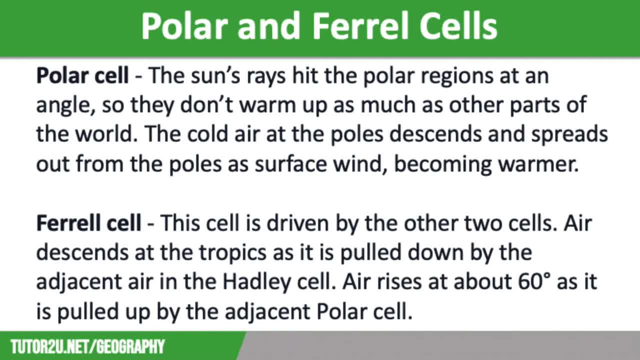 These extend from between 60 and 70 degrees north and south to the poles. The sun's rays hit the polar regions at an angle, meaning they receive less concentrated solar radiation and they don't warm up as much as other parts of the world. The cold air at the poles descends, meaning there is 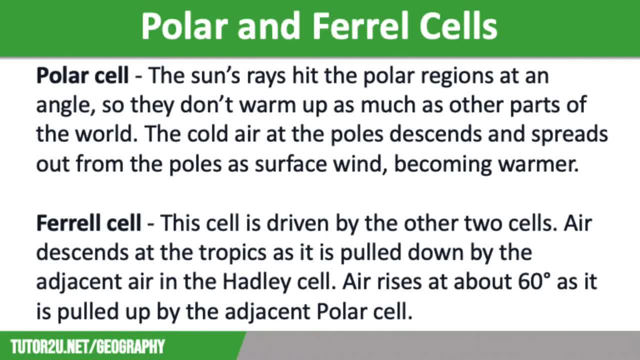 no condensation and rain. This cold air spreads out from the poles as surface wind becoming warmer At around 60 degrees, this warm air rises, leading to clouds and rain. This air will then flow back to the poles. The ferrule cell is found in the middle and is driven by the other two cells. 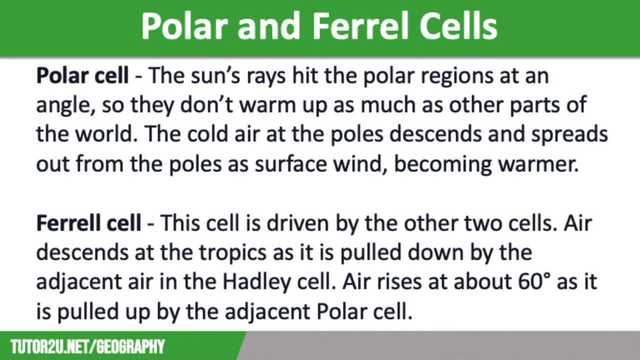 Air descends at the tropics as it is pulled down by the adjacent air. in the Hadley cell, Air rises at about 60 degrees as it is pulled up by the adjacent polar cell, Air converges at low altitudes to ascend along the boundaries between the cool. 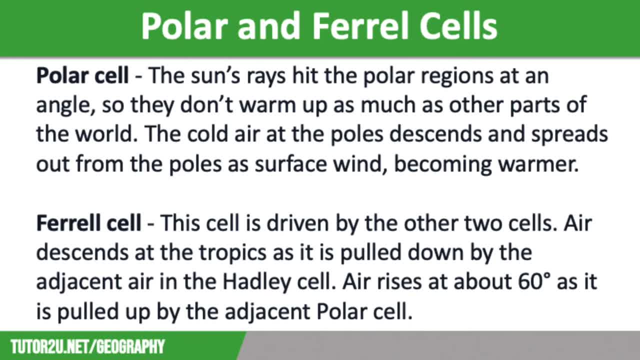 polar air and the warm subtropical air that generally occur between 60 and 70 degrees north and south of the equator. This often occurs around the latitude of the UK, which gives us our unsettled weather. The circulation within the ferrule cell is completed by a return flow of air at high. 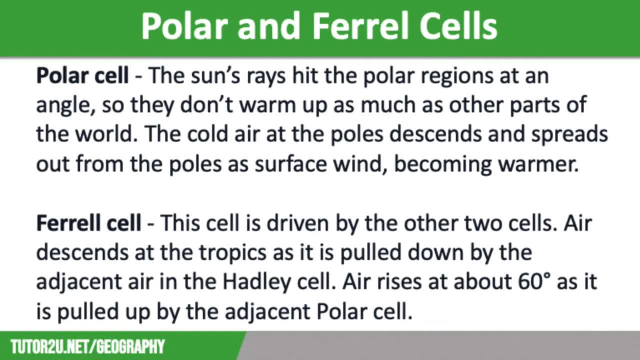 altitudes towards the tropics. This is where it joins sinking air from the Hadley cell. The ferrule cell moves in the opposite direction to the other two cells and acts like a gear. In this cell, the surface wind will flow from a southerly direction in the northern hemisphere. 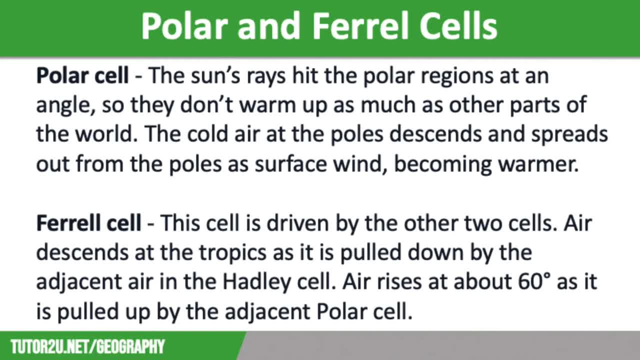 However, the spin of the wind will flow from a southerly direction. in the northern hemisphere, However, the spin of the wind will flow from a southerly direction. in the northern hemisphere, The spin of the earth induces an apparent motion to the right in the northern hemisphere. 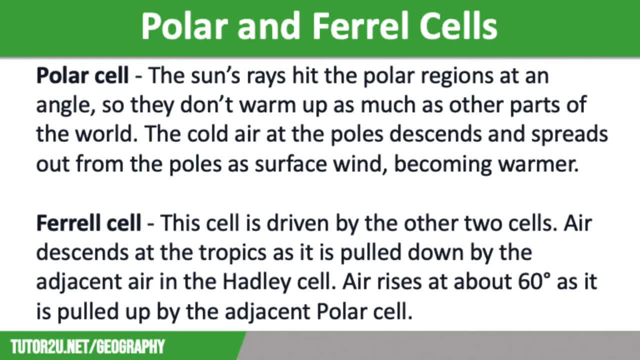 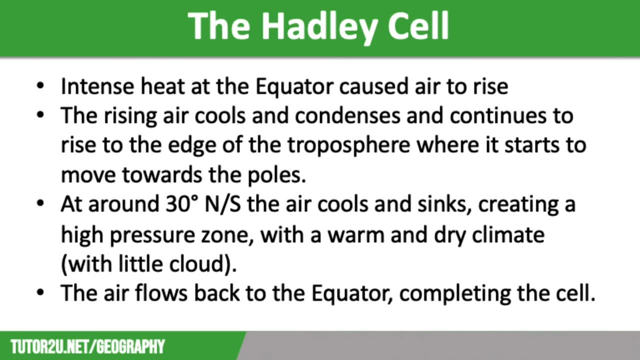 and left in the southern hemisphere. This deflection is caused by the Coriolis effect and leads to the prevailing westerly and south westerly winds often experienced over the UK. The Hadley cell is a cell that you do need to know about. 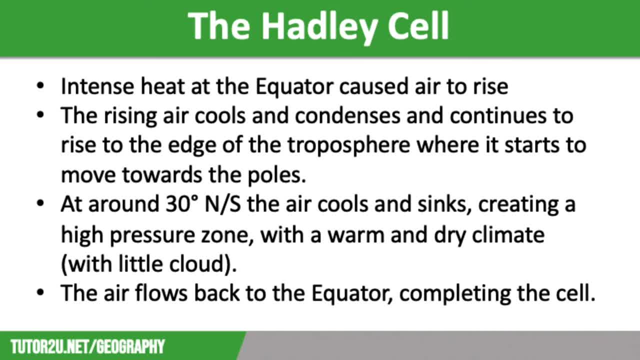 The sun shines intensely on the equator, heating the land. This in turn heats the air, which rises, creating a low pressure zone at lower levels. The rising air cools and condenses, forming towering cumulonimbus storm clouds. The air continues to rise to the edge of the troposphere where it starts to move towards. 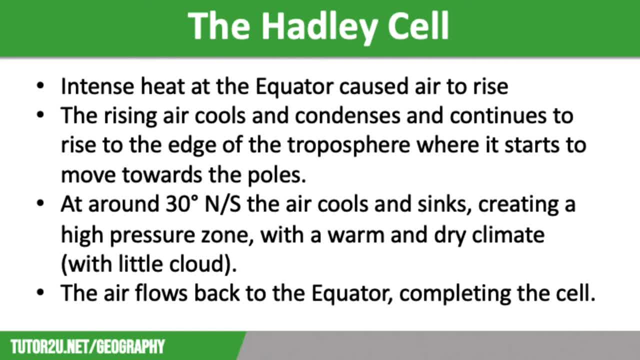 the poles north or south. At around 30 degrees north and south, the air cools and sinks, creating a high pressure zone, A warm and dry climate with little cloud, Typically where deserts are found. Surface winds take the air from the tropics back to the equator, completing this cell. Within the Hadley cells, the tradewinds blow towards the equator. They then ascend near the equator as a broken line of thunderstorms, which form the intertropical convergence zones, or the ITCZ, At a depth of around 30 hectares, with about 995m2 of atmosphere. 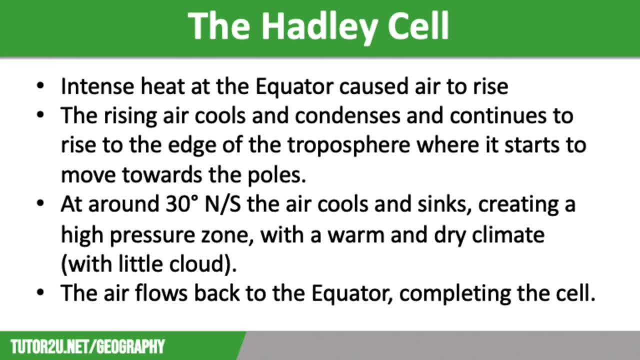 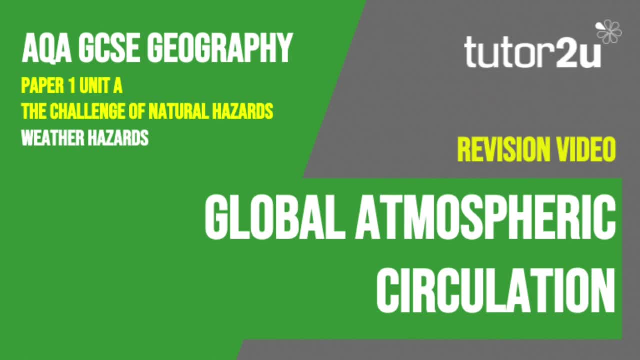 From the tops of these storms, the air flows towards higher latitudes, where it sinks to produce high-pressure regions over subtropical oceans and the world's hot deserts, such as the Sahara in northern Africa. That concludes this 2-2-2-U revision video focusing on global atmospheric circulation. Thank you for watching.